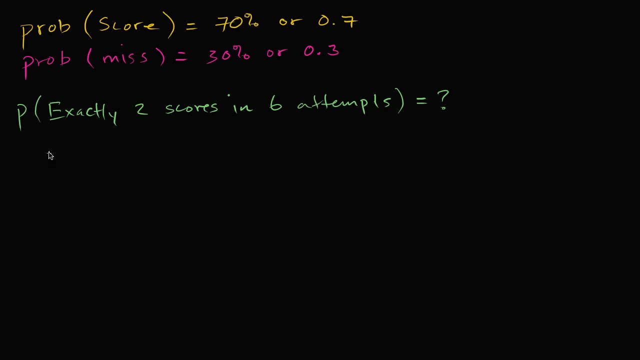 you could get, you could make the first two free throws, So it could be score, score, and then you miss the next four, So score, score, and then it's miss, miss, miss and miss. So what's the probability of this exact thing happening? 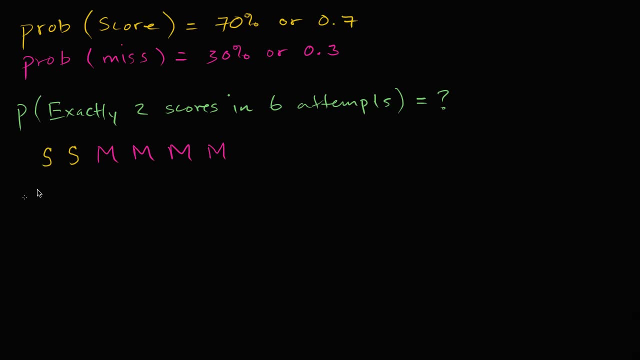 This exact thing. Well, you have a 0.7 chance of making of scoring on the first one, Then you have a 0.7 chance of scoring on the second one, And then you have a 0.3 chance of missing the next four. 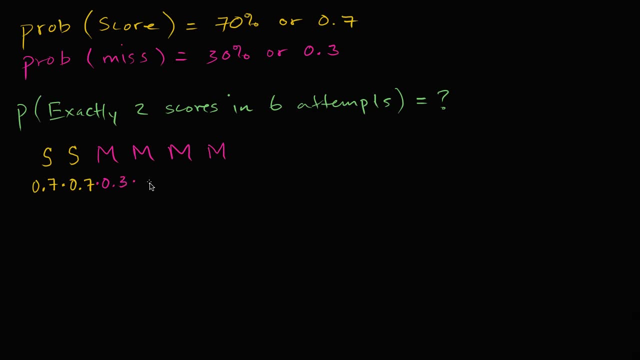 So the probability of this exact circumstance is going to be what I'm writing down, And hopefully you don't get the multiplication symbols confused with the decimals. I'm trying to write them a little bit higher. So times 0.3.. And what is this going to be equal to? 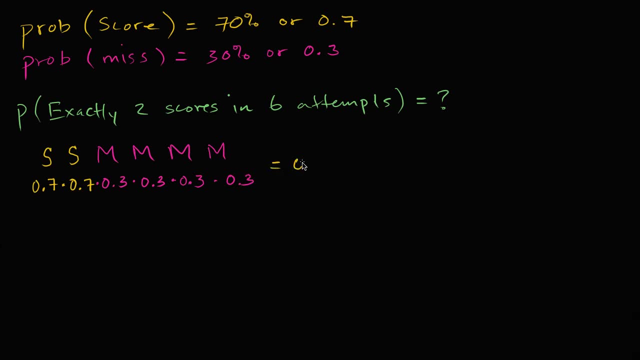 Well, this is going to be equal to. this is going to be 0.7 squared times 0.3, times 0.3 to the one, two, three, fourth to the fourth power. Now is this the only way to get two scores in six attempts. 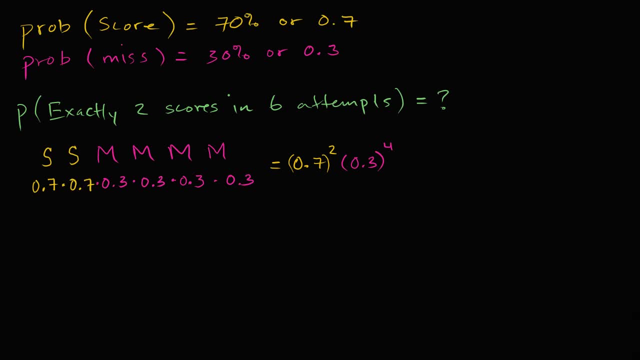 No, there's many ways of getting two scores in six attempts. For example, maybe you miss the first one, the first attempt, and then you make the second attempt. you score, then you miss the third attempt and then you, let's say, you make the fourth attempt. 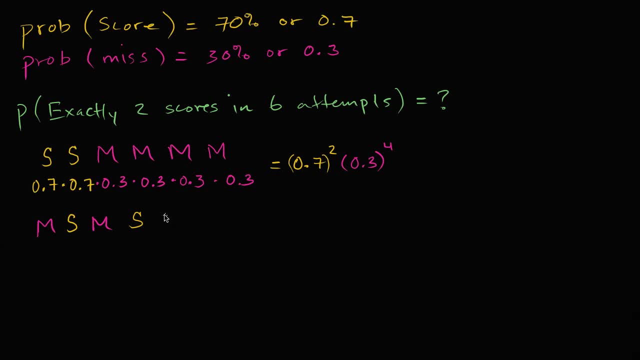 and then you miss the next two. So then you miss and you miss. This is another way to get two scores in six attempts. And what's the probability of this happening? Well, as we'll see, it's going to be exactly this. 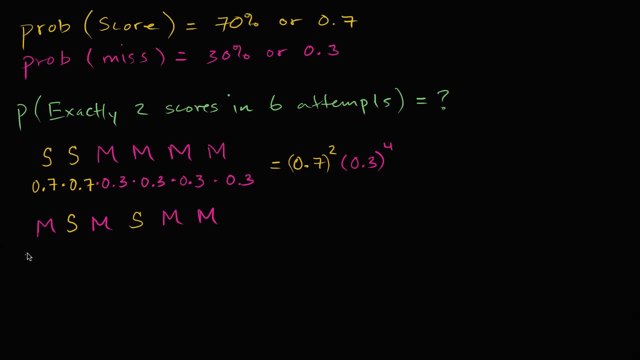 it's just we're multiplying in different order. This is going to be 0.3 times times 0.3, 0.7,. you have a 30% chance of missing the first one, a 70% chance of making the second one. 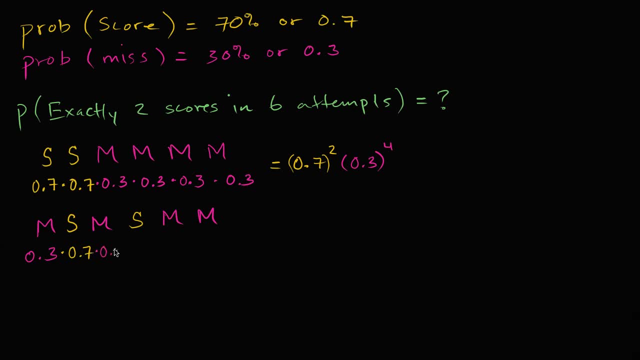 and then times 0.3, 30% chance of missing the third times, a 70% chance of making the fourth times, a 30% chance for each of the next two misses. If you wanted this exact circumstance, this exact circumstance. 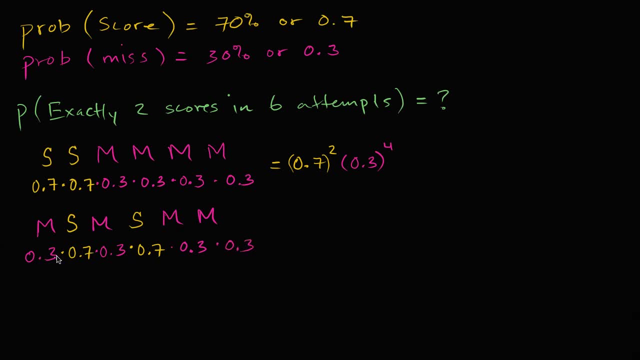 this is once again going to be 0.7,. if you just rearrange the order in which you're multiplying, this is going to be 0.7 squared times 0.3 to the fourth power. So for any one of these particular ways, 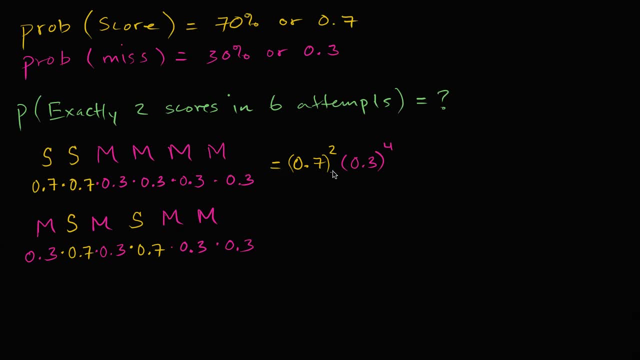 to get exactly two scores in six attempts. the probability is going to be this. So the probability of getting exactly two scores in six attempts, well, it's going to be any one of these probabilities times the number of ways you can get six scores. 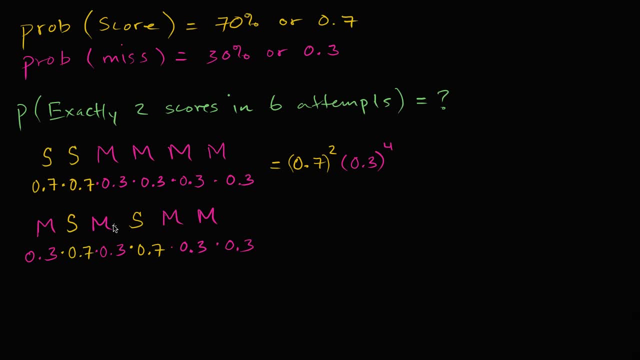 times the number of ways you can get two scores in six attempts. Well, how, if you have, out of six attempts, you're choosing two of them to have scores? how many ways are there? Well, as you can imagine, this is a combinatorics problem. 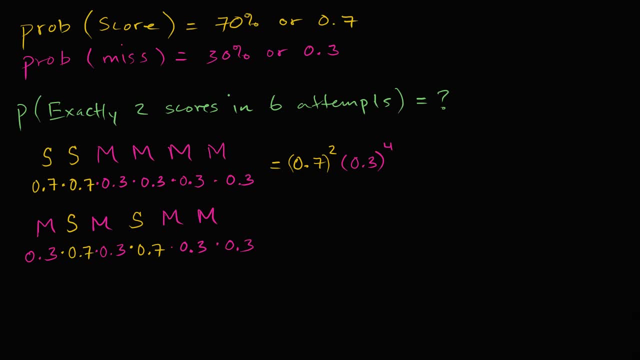 So you could write this. as you could write this, and let me see how I could- you're going to take six attempts, so you could write this as six. choose, or we're trying to, if you're picking from six things. 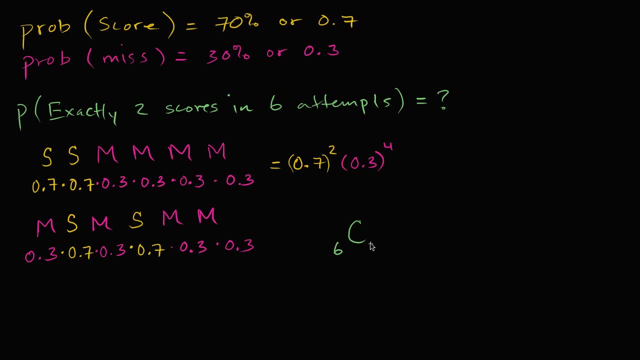 your six attempts and you're picking two of them, or two of them are going to need to be made if you want to make meet these circumstances. This is going to tell us the number of different ways you can make two scores in six attempts. 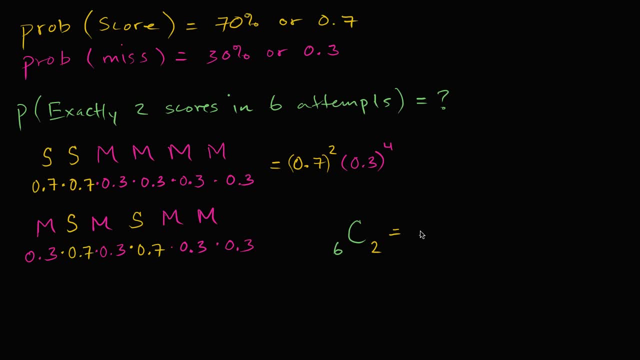 and of course, we can write this in kind of the binomial coefficient notation. We could write this as six choose two, six choose two, and we could just apply the formula for combinations, and if this looks completely unfamiliar, I encourage you to look up combinations on Khan Academy. 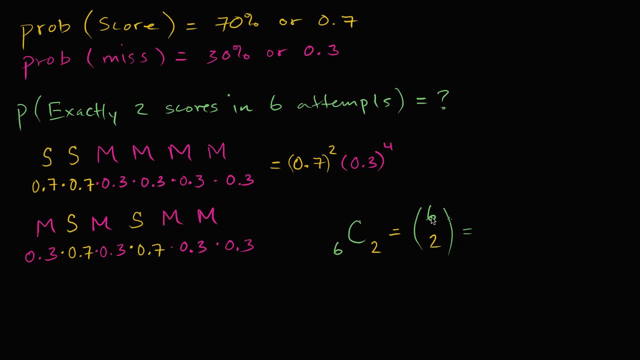 and we go into some detail on the reasoning behind this formula, It actually makes a lot of sense. This is going to be equal to six factorial over two factorial over two factorial times six minus two factorial, So six minus two, six minus two factorial. 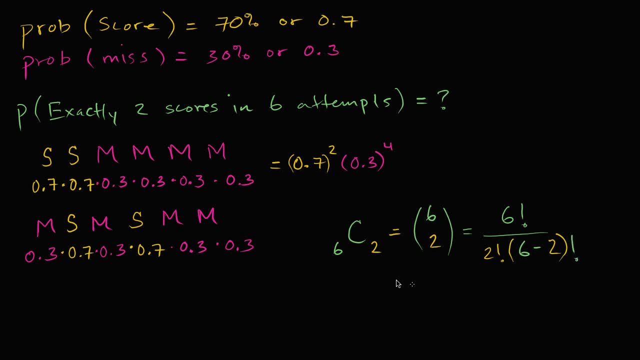 I'll do the factorial in green again: Six minus two factorial. and what's this going to be equal to? This is going to be equal to six times five times four times three times two, and I'll just throw in the one there. 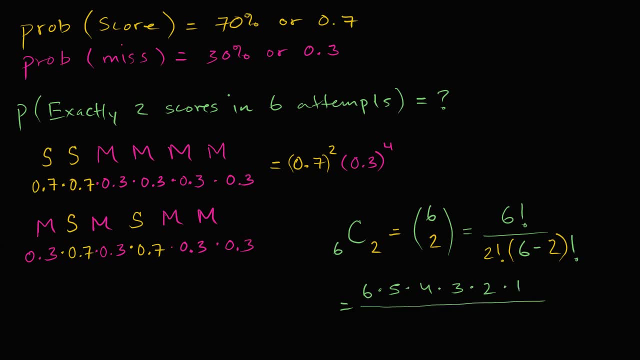 although it doesn't change the value. over two times one, over two times one. and six minus two is four, so that's going to be four factorial. So this right over here is four factorial. so times four times three times two times one. 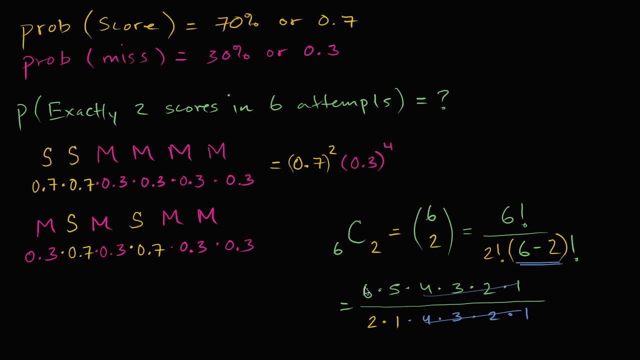 Well, that and that is going to cancel. and then let's see: six divided by two is three. so this is 15. There's 15 different ways that you could get that. you could pick two things out of six, I guess is one way to say it. 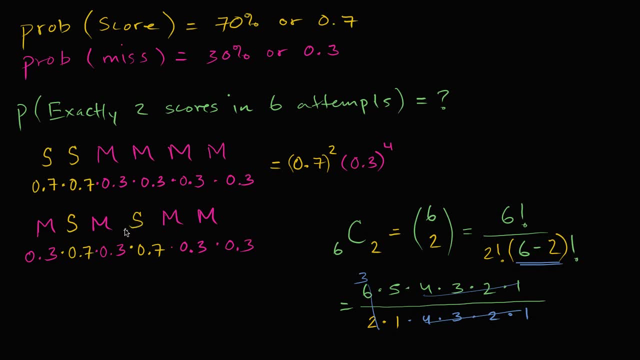 Or there's six, there's 15, did I say 16?? There's 15, the sixes and the fives. there's 15 different ways that you could pick two things out of six. Or another way of thinking about it is: 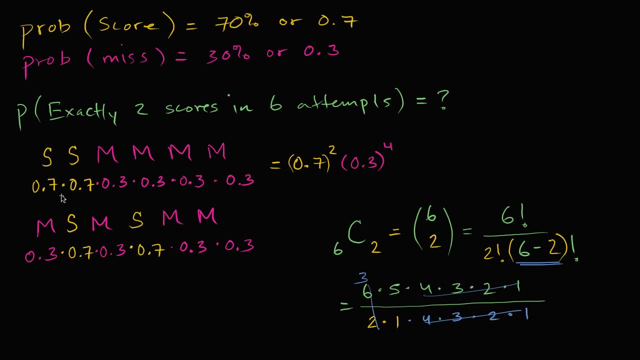 there's 15 different ways to make two out of six free throws. Now the probability for each of those is this right over here, So the probability of exactly two scores in six attempts. well, this is where we deserve a little bit of a drum roll. 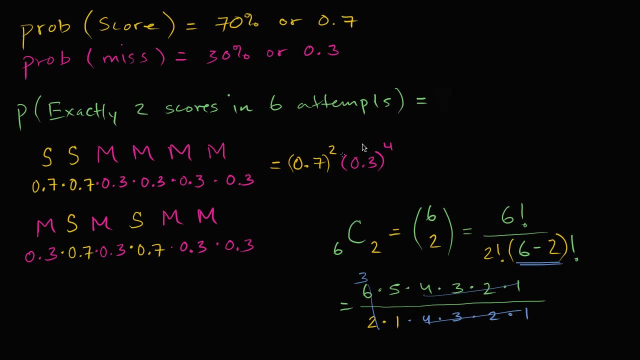 this is going to be, this is going to be six. choose two times 0.7,. 0.7 squared, that's, this is two, two. you're going to make two, you're going to make two, and then it's 0.3,. 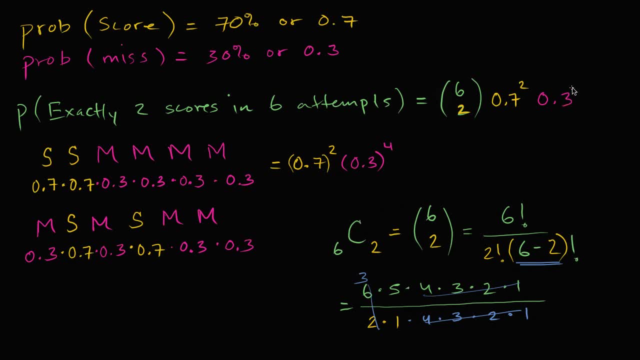 0.3 to the 0.3 to the fourth power. Now notice these will necessarily add up to six. So if this right over here was a three, then this right over here would be a three, and then this would be six minus three. 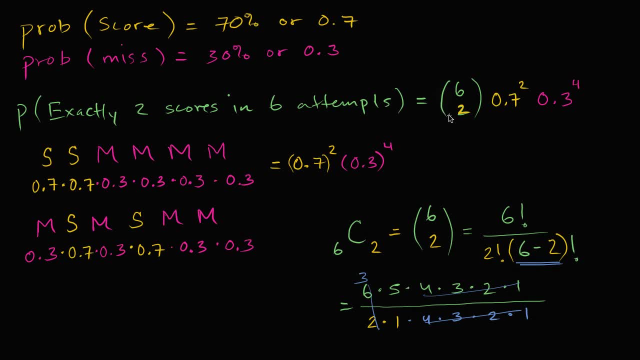 or three right over here. And now, what is this value? Well, it's going to be equal to. it's going to be equal to: we have our 15, three times five. so we have this business right over here. it's going to be 15 times. 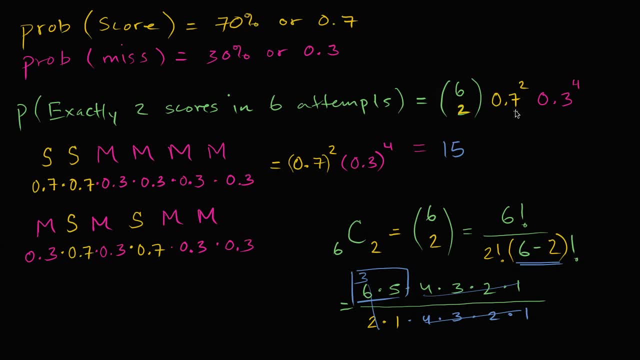 times. let's see 0.7 times. 0.7 is going to be times 0.49, and let's see: three to the fourth power would be 81,. three to the fourth power would be 81,, but I'm multiplying four decimals. 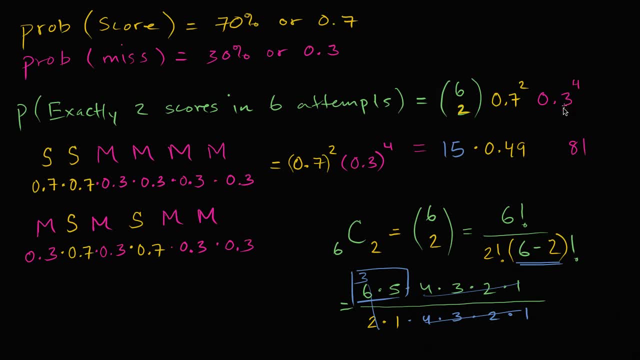 each of them have one space to the right of the decimal point. so I'm going to have- this is going to- I'm going to have four spaces to the right of the decimal, so 0.0081.. So there you go. 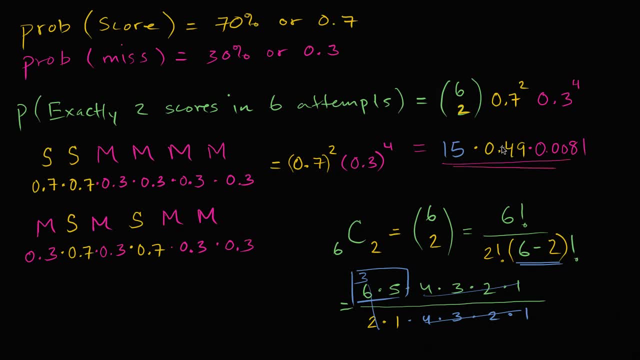 whatever this number is- and actually I might as well get a calculator out and calculate it- So this is going to be, this is going to be. so it's 15 times 0.49, times 0.0081, and we get 0.59,. 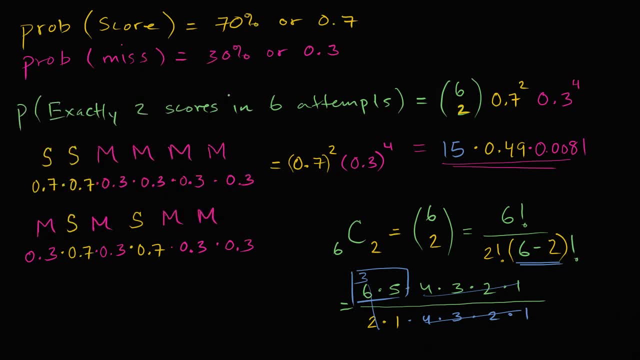 0.99535.. So this is going to be equal to: let me write it down, and actually maybe I'll. I wish I had a little bit more real estate right over here, but I'll write it in a very bold color. 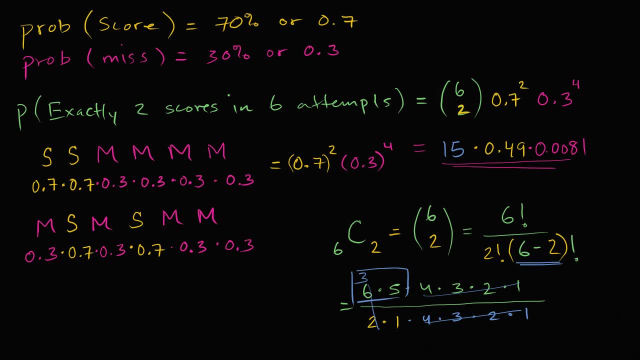 This is going to be. actually. I'm kind of out of bold colors. I'll write it in a slightly less bold color. This is going to be equal to 0.05935. 0.05935, or we could say this is approximately. 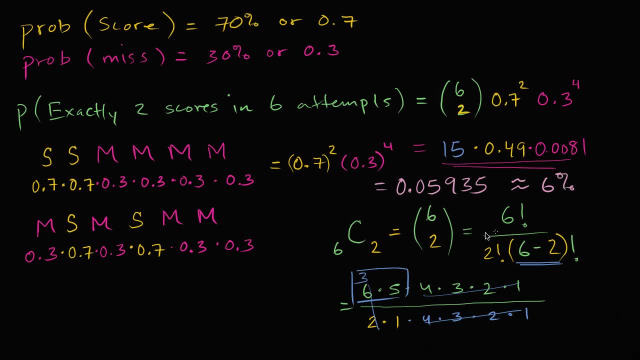 if we round to the nearest percentage, this is approximately a 6% chance- 6% probability- of getting exactly two scores in the six attempts. I didn't say two or more, I just said exactly two scores in the six attempts And actually it's a fairly low probability. 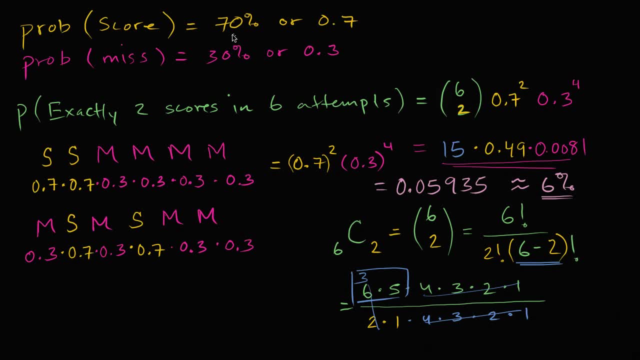 because I have a pretty high free throw percentage. If someone has this high of a free throw percentage, it's actually reasonably unlikely that they're only going to make two scores in the six attempts. 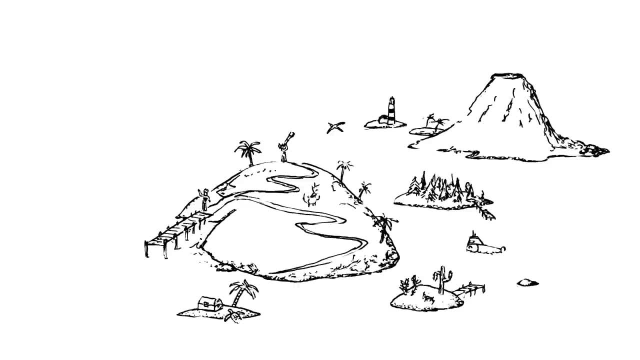 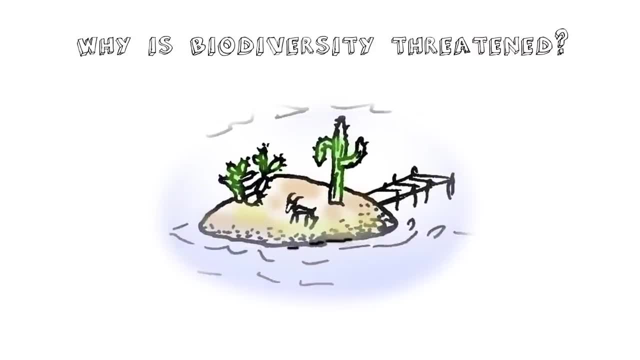 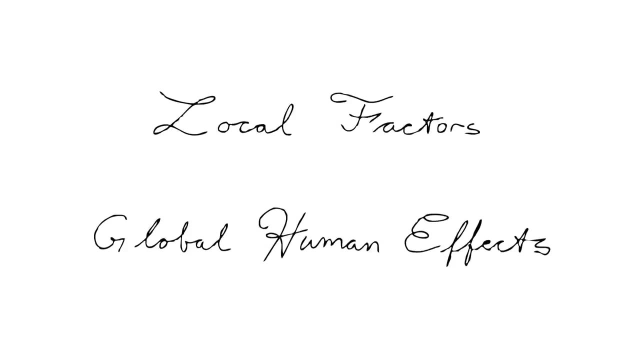 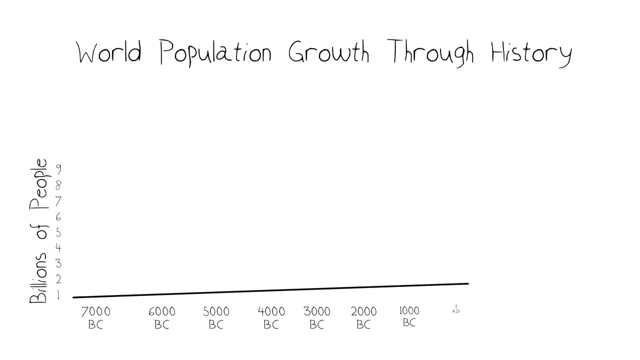 Why is biodiversity threatened? We're going to talk about something that we'll call local factors as opposed to more global human effects, But before we go into some of those, we really need to talk about the fact that the human population is growing fast. In 2014,, the estimate was just.